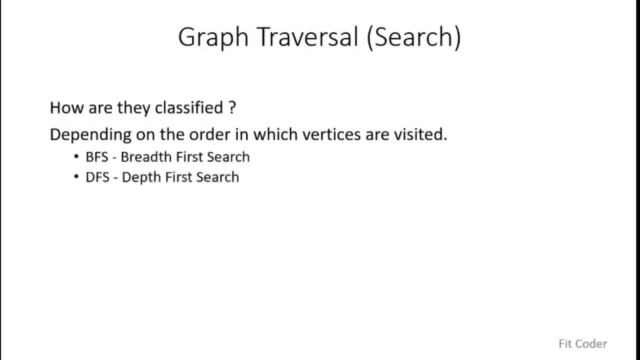 on the order on which vertices are visited. so there are basically two types of graph algorithm, which is called the first one, which is called the breadth first search, and the second is known as the next one, which is the breadth first search. so i have split this into two videos. in the first 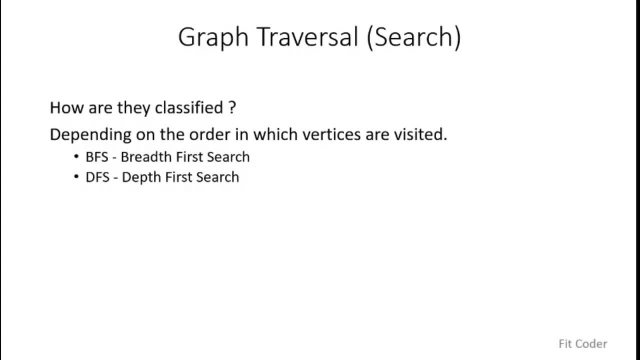 video i will be discussing breadth: first search. what are the applications of it, what is the algorithm and how we can implement it. so these things will cover this video, and in the next video we'll discuss the dfs. so now let's discuss what we meant by breadth: first search the breadth. 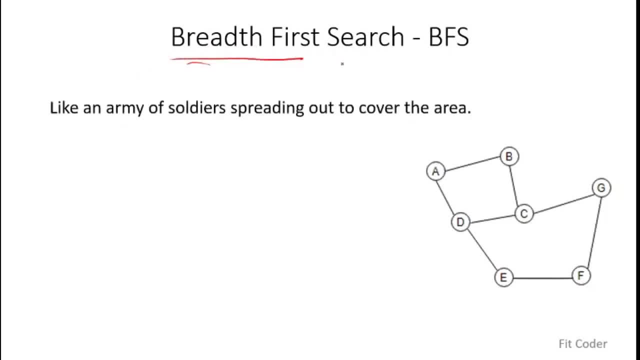 first search is like an army of soldiers which is spreading out to cover the area. what we mean by that is, let's say we are in a battlefield and we come across a junction which has four directions. explore all the four directions to us so as to find the enemies. so what we do is we send some. 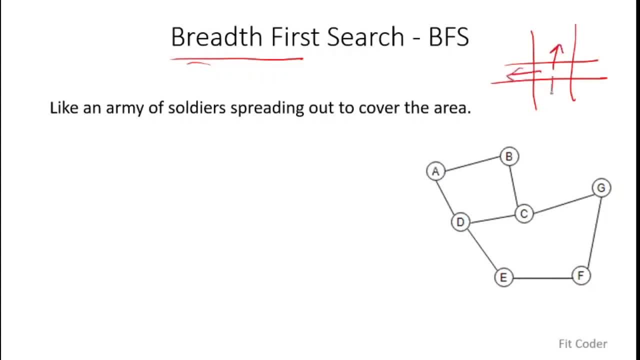 soldiers of the army in this direction, some in this direction, some in this and some in this. so we have spread out all the army to cover the entire area. so that is the basic essence that we do in breadth: first search. one important term to note here is that we have to explore the graph. 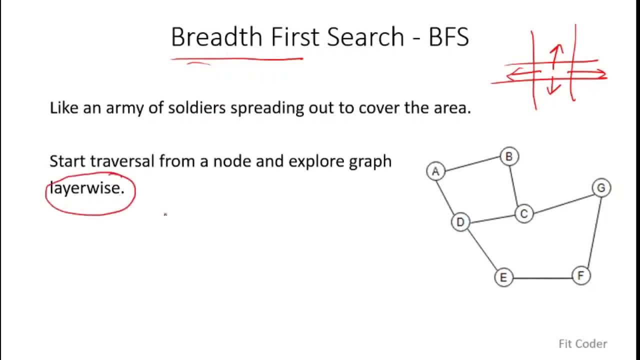 layer wise. so now let's try to understand what we mean by layer wise. so we have this graph which has seven nodes, and let's assume that we are starting from a. so basically we have to reach g, f, e, d, c, b from a. so one easy way to understand is: let's assume that all the edges have weight one. 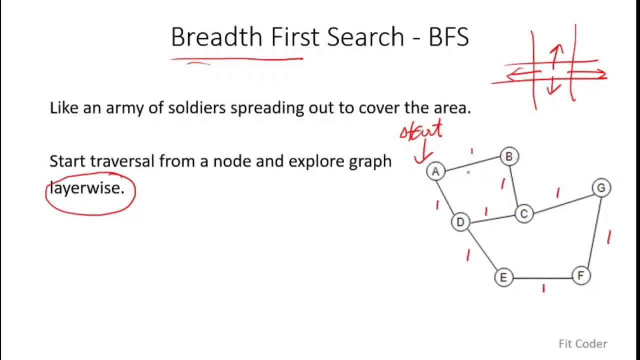 and now let's try to find the distance of each of these nodes from the vertex or from the starting point. a, so this edge weight is a, so this node is a distance one. b is also a distant one. c: you will either reach from b or from d, so its distance is two. g distance is three. 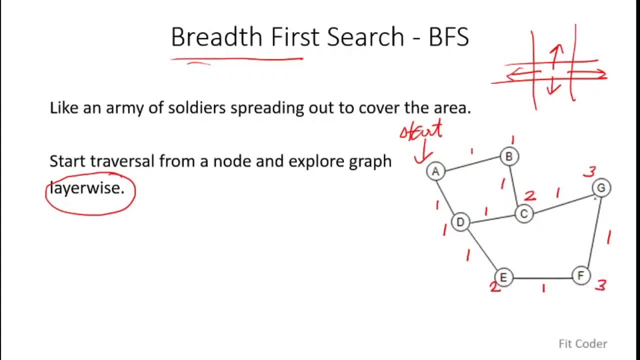 e, distance is two, f is at three. so these are the distances which are there from starting point a. we have started from here. we have to explore all the graph. so when we say layer wise this, so in each layer we'll explore the nodes that are at equal distance from the starting point. 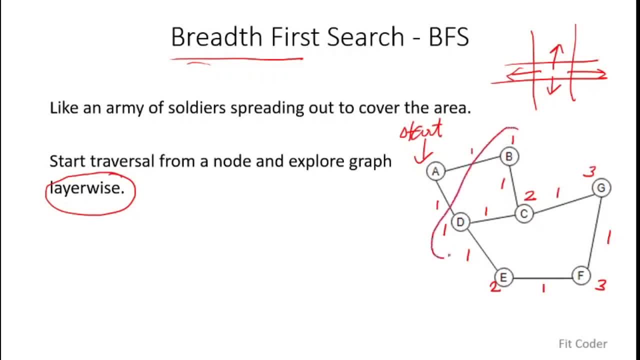 so b and d are at distance one. so in the first layer we'll discover these two nodes after discovering these. so c and d are at a distance two. this, this is the first layer and this is the second layer, and in third layer, g and f. so they both are at the equal distance. this will be explored in third. 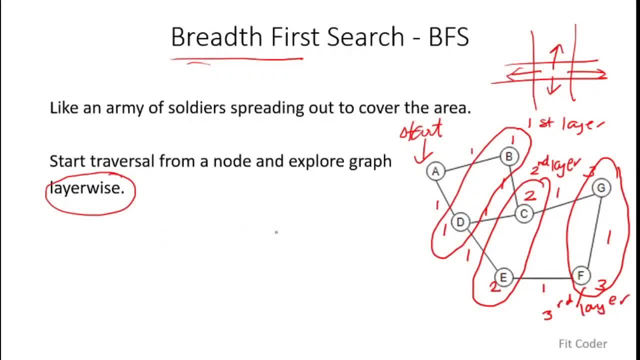 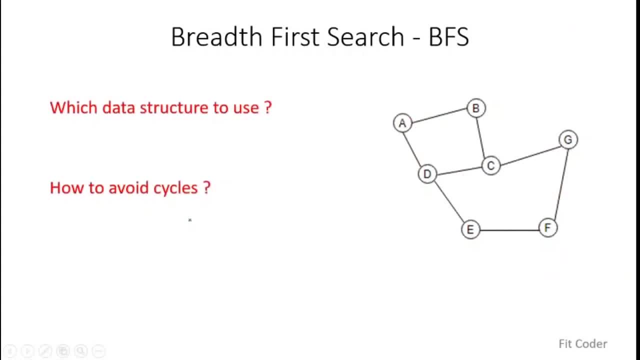 layer. so when we say layer wise, so that means we have to explore the graph depending on the equal distance from the starting point. okay, now when we are implementing bfs, there are two important questions that we face. one is the: which data structure should we use to implement bfs? so now, as 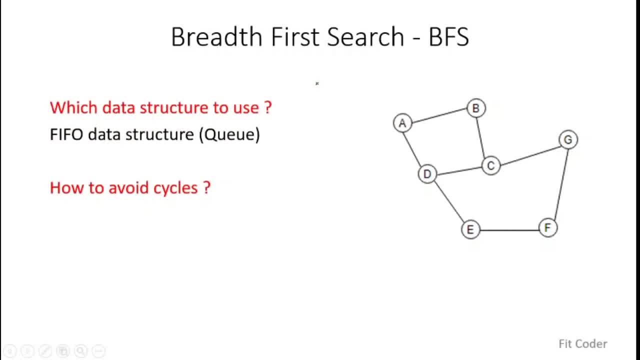 we see that the data structure that has to be used is fifa data structure, which is a q. but why fifo is bfs. so in bfs we pick a start node. so this is the start node and we explore in all the possible directions. and whichever node we discover, first we have to explore it. and important property of fifo. 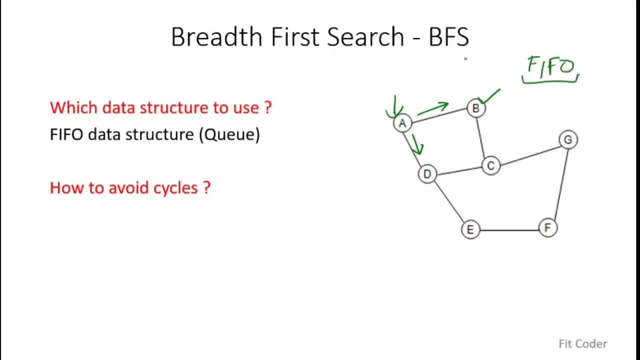 is first in, first out. so this is in alignment with how we are going to implement bfs. now, people often confuse between bfs and dfs. so bfs uses q and dfs uses stack. so when we are talking about breadth, we generally relate it with something that is horizontal, and when we are talking about the, 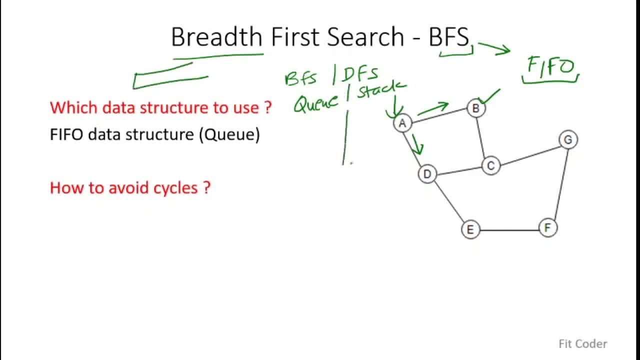 horizontal and when we are talking about depth, that is generally related with height, so breadth, which is more aligned with horizontal, so that is more rated with q, and depth, which is more related with stack, because whenever we say stack we mean like a stack of books or a pile of books, so that 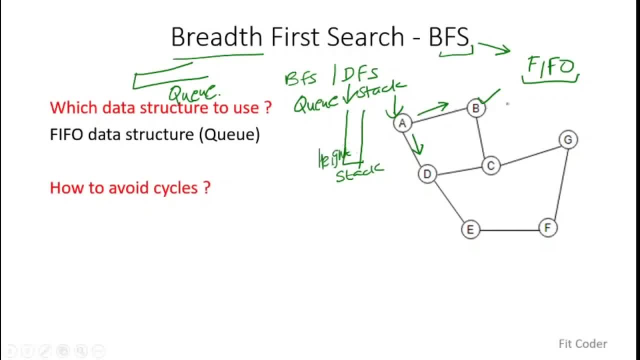 is more in relation with height. another funny way to remember is: so just remember the word barbecue. so how people relate is this. so b is short form for bss and q means data structure. q use q. so this is also funny way which people use to remember which data structure has to be used for. 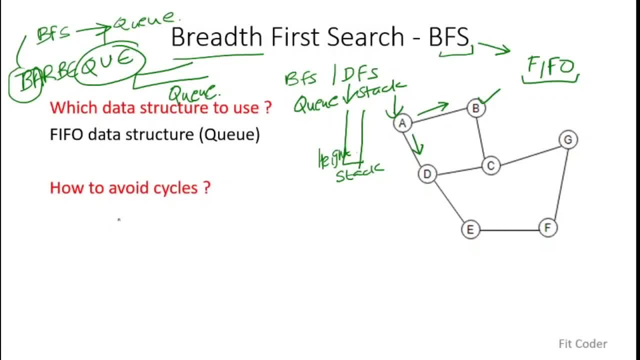 bfs. so now, once we have this concept clear, that q is to be used for bfs, then the other important question arises that how are we going to avoid cycles? so let's say, in this one we are starting with a, explore both these nodes, b and d. so now, from b, the adjacent node is c, but for d we are. 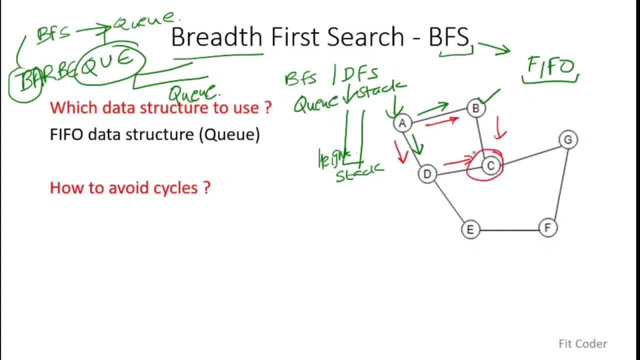 just notice c. so once you have discovered also, there is a tendency to go back to b. if you do this, doing graph traversal, you have to avoid cycles. so how we can do that is we need to keep track of the nodes that we have visited. we can keep an array or a hash map that will keep track of which. 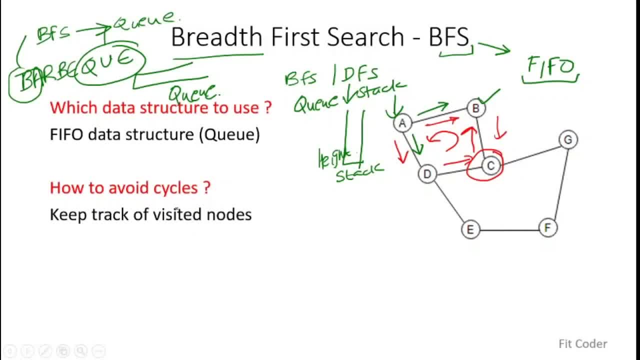 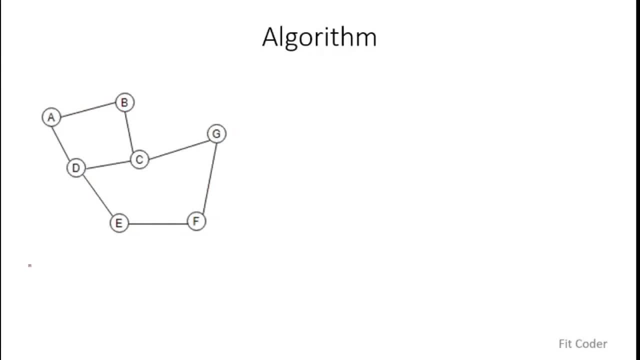 of the nodes you have visited, so you do not end up in a loop. so these are the two important things that we have to keep in mind when we are going to implement bfs. so now let's discuss the algorithm that is used for bfs. so we discussed that we need to have a data structure, q- and also we need to 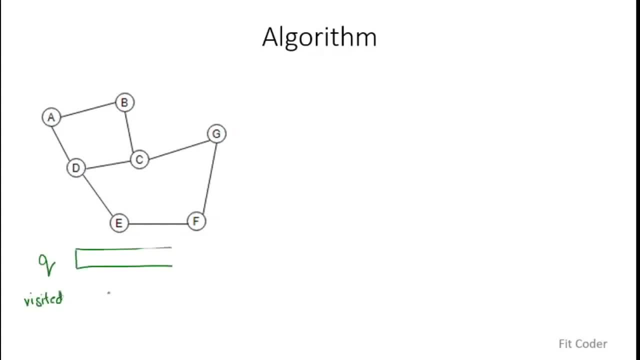 keep track of which of the nodes are listed. so i'll keep a listed array. so we have seven nodes here, so i'll keep an array of seven nodes: e, f, g, so seven are the vertices. so initially all of them are empty, which means that none of them has been listed. and let's say that a is the start node. 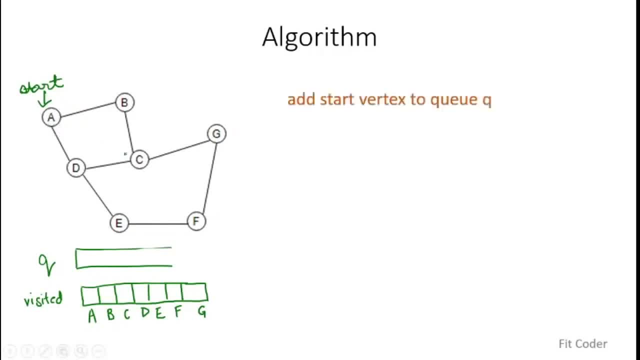 so from a we have to explore this entire graph. so the first step is add start vertex to q. so start vertex is a, so we'll add a to the q. this is the first step. second step is mark start as listed. we mark them as listed. so we did a check here. so we did a check here. so we did a check here. 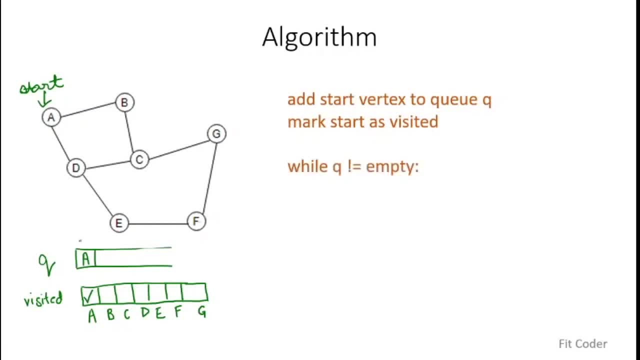 a is listed now. then we have to check while q is not empty. so q is not empty, q has element a in it. then we have to check what is the front of the q. so front of the q is v, so this is a currently. so when we say front of the q, this operation means that we have to dequeue the q also. 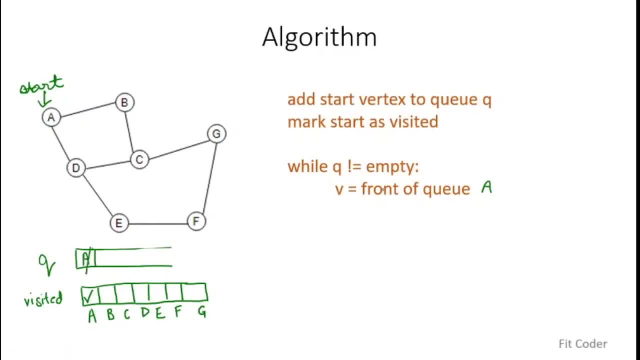 so we dequeue the q and let's keep track of the output. so whenever we dequeue we'll add it to the output. this is the output: a. then we check that for each adjacent vertex a, v of v. so v was a. the adjacent vertices for a are b and d. so we have to run this. 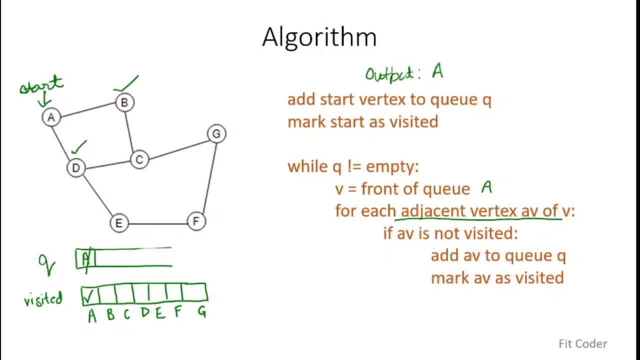 for both of these elements, b and d. so if av is not listed, add av to q. so first time the additional vertex let's pick as b, so b is not wasted because there is no tick box here. so add b to q and mark a visit to. then again we come to the next addition vertex of. 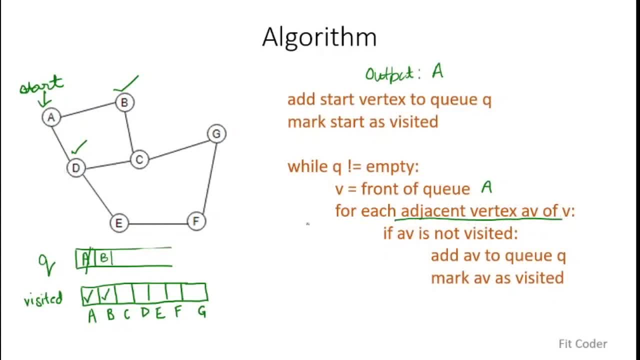 v, which was a. it next original vertex was d. we check if d is not wasted, not listed, so we add d here and also we mark d as listed. then again this loop is done. we come again here while q is not empty. so q is not empty because it has two elements, b and d. so we pick. 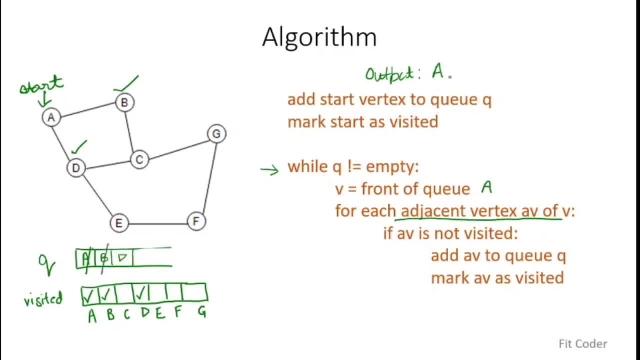 the front of the q. so front of the q is b, so output becomes a, b for each adjacent vertex of b. we have to run this loop. so adjacent vertices of b are a and c. so we check if av is not listed, so first comes a. but a is already listed because we have marked entry. so we have to skip a. 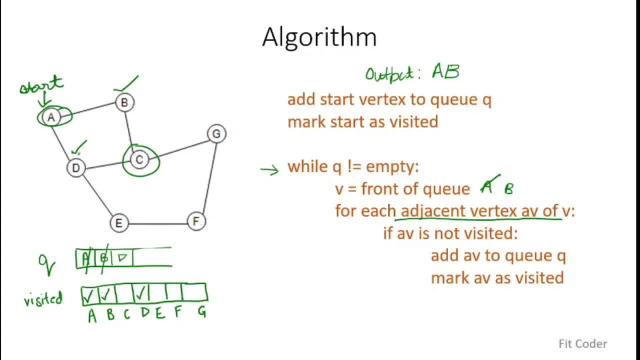 so here we have avoided cycles, because if we have again processed a, then we will always run in this loop. but since we have marked entry of a as listed, so we are skipping this loop. so the next adjacent vertex of b is c. so we add c to the q and we mark c as listed. then we again come here. q is not empty. 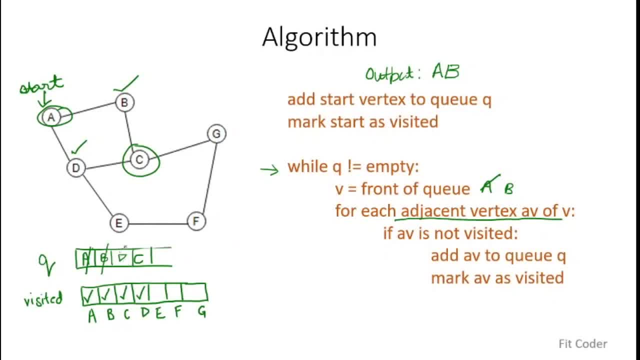 because it has two elements. we pick the front of the q. the front of the q is d, so we add it to the output and b is here d. adjacent vertices of d are a, c and e. but a and c are already listed because we have marked their entries. so we have to process. 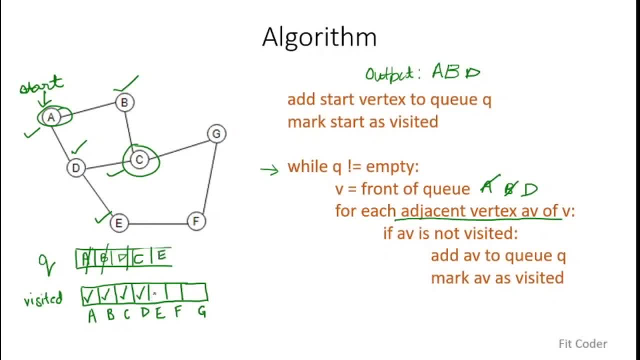 e. so we'll add e to the q and we'll mark it as a listed. next we again come here, while q is not empty. so the first element of the front of the q is c. so we'll add c to the output and we b becomes c. 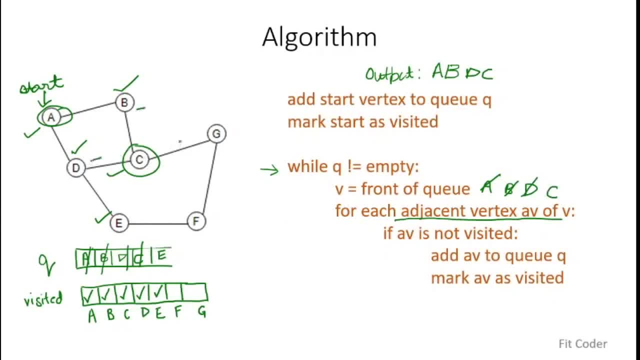 adjacent vertices of c are b, d and g. but b and d are already listed, so we add g to the q and we mark d this time again, because q is not empty. so we have suspended. all the adjacent nodes of c are processed. then we again come here while q is not empty. so q is not empty. the front of q is e, so we 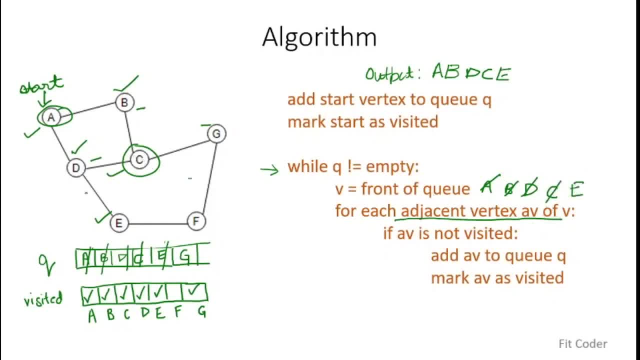 pick e here and mark e in the output. so v is now e. dissonant nodes of e are d and f. but d is already processed because its entries mark. so we pick f and we append f to the q and it mark its entry as 1.. then all the adjacent vertices are possessed. 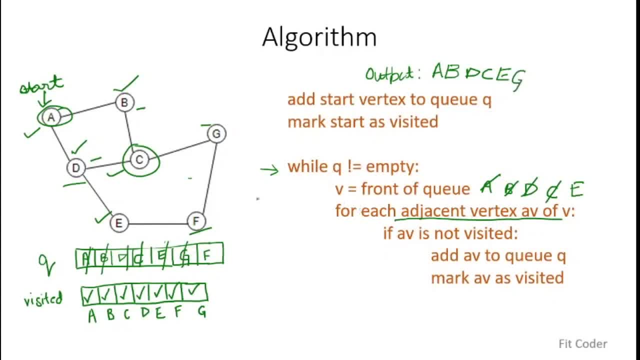 q is not empty. we pick g, check adjacent vertices of g. adjacent vertices of g are c and f. but c and f both are processed, so we do not do anything here. we come again here while q is not empty. so q has element f. now we pop f and adjacent vertices: we check. adjacent vertices are e and g. 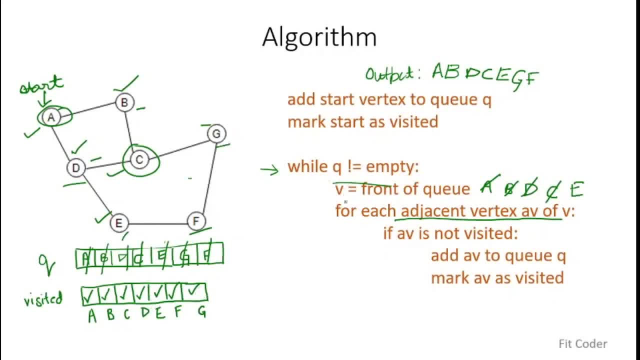 but e and g, both are processed, so we do not do anything. and next time we come here the q is empty. so we get this as output: a, b, d, c, e, g, f. so this is the bfs traversal of this graph. so if we check also the distance theory that i have told earlier, so both of these are in first layer, then both of 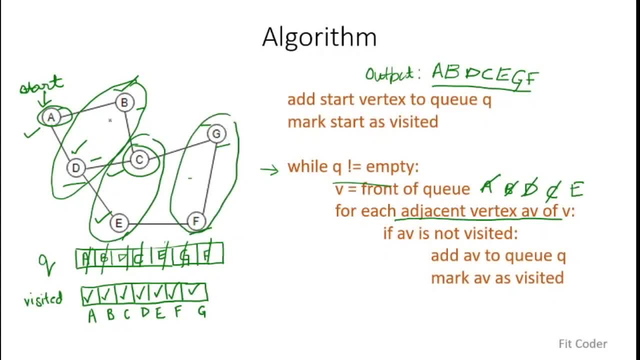 these are in second layer, then these are in third layer. first is the a, then b d, c, e g f. b d, c, e g f. so this is how this traversal has been done. so this is one of the traversal of this graph. so if you see here when we started, 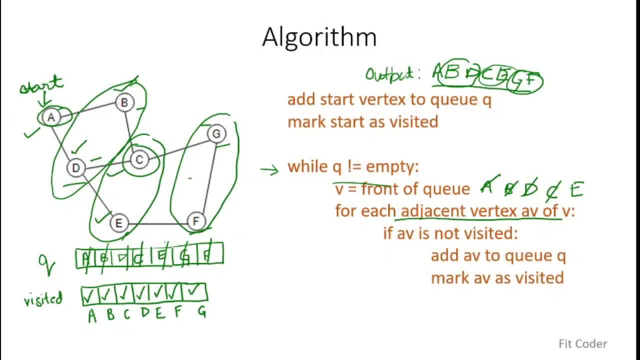 spread out from a, so we have picked b first. so if we enter d in the q first, so because d and b both are equidistant, so if we enter d in the q first, so we'll. this order will be a little different. there can be multiple bfs traversals of the same graph, so i've listed down some traversals. 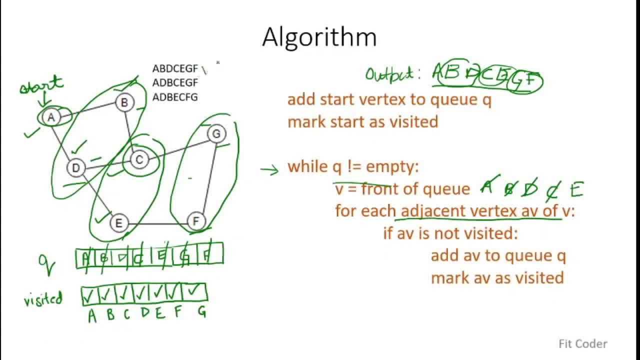 so first one: we traversed a, b, d, c, e, f, g, f. second one will be when d and b are interchanged, because we can traverse any one of these. so if we do that, then we'll get this one. now, if we traverse d and b, then also this c and d can be interchanged, so we can get this graph also. 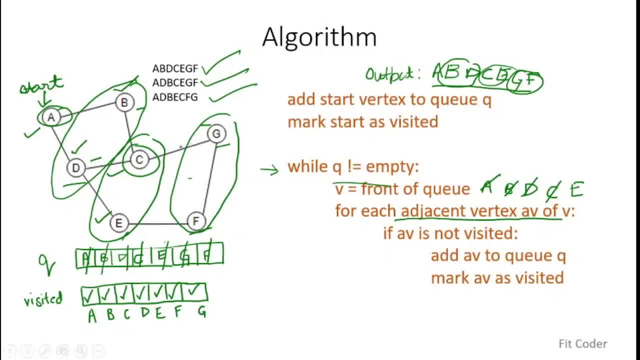 so there can be multiple variations of bfs traversal of the same graph, but all the nodes that are equidistant from each other will be explored, because then the nodes that are far away from them? that is the basic essence of bfs algorithm. so one important thing to note here is: 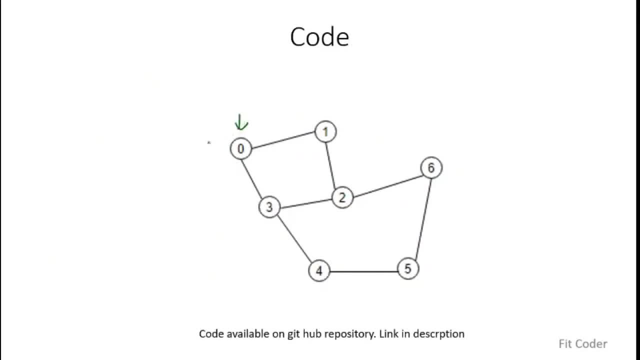 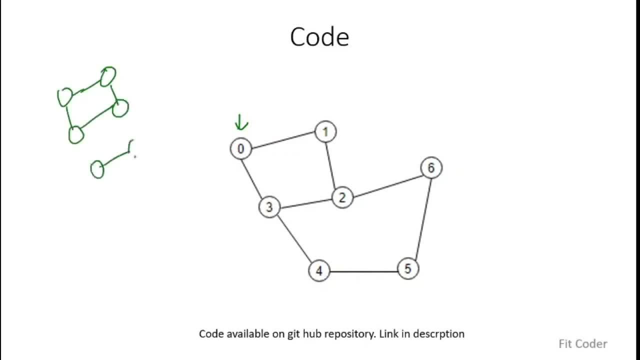 disconnected, let's say, if the graph is disconnected. let's say: if the graph is disconnected, let's say, you are given a graph like this: this is the graph that you have and you start your traversal from node a. so in this case, you will only end up traversing nodes like this: a, b, c, d, but ef will. 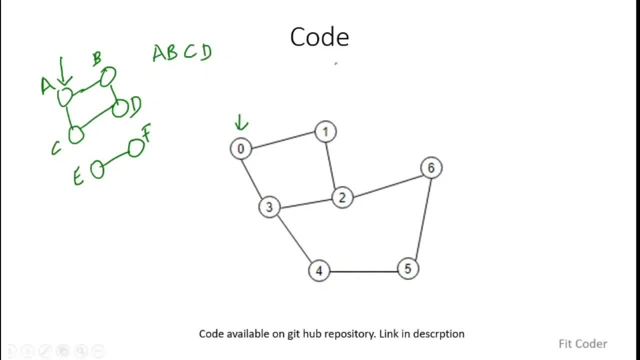 not be covered because there is no edge connecting them. so in this case, what you do is: so you have this listed array, so which have entry for all these nodes, and a, b, c, d will be marked after this iteration and ef is still left. so what you do is whatever nodes are left after this queue is empty. 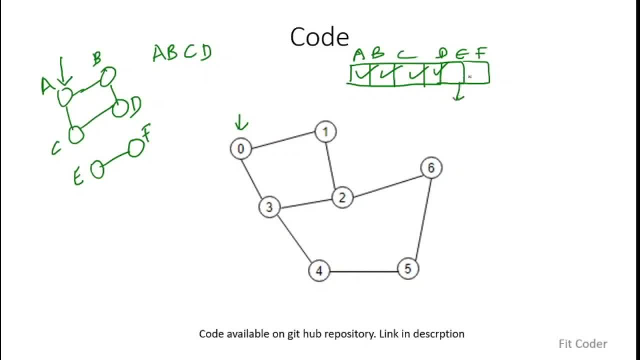 so you pick that node and you do a bfs traversal again from that. so you will pick this e and this will be the new start vertex and you will do a bfs traversal from there. so a, b, c, d and e, f, so this is the complete traversal. 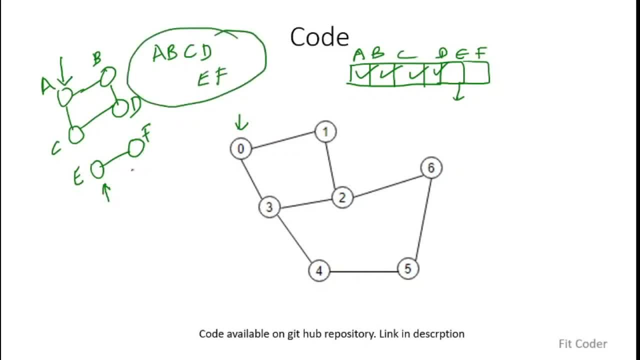 of the graph. so you visit each node. so this you have to take care. you're not sure whether the graph is connected or not. then you do a bfs traversal for all individual components of the graph. now, once we have understood the concept behind bfs, let's try to implement this. i'll be. 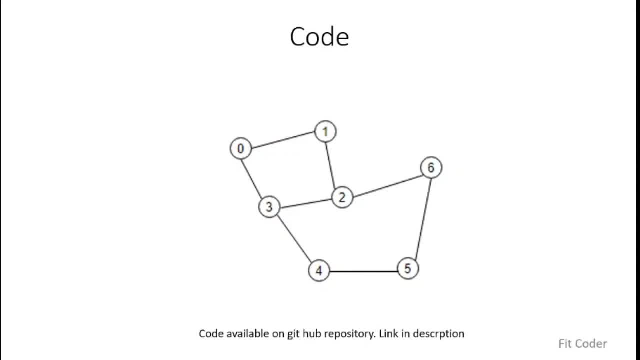 using c plus plus, and all the code that i'll be using will be available in my github repository. link of that is in the description. the example i'm using is the same one which you've discussed, just that instead of alphabets i have numbered them from 0 to 6, so they're total seven vertices. 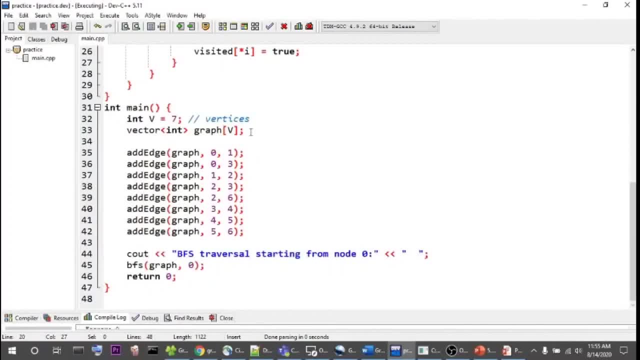 let's now jump into the code. so first i have created a graph representation for my adjacency list. i've added all the edges that are shown in the diagram. then i call this function bfs, where i pass the graph and the starting vertex. i am traversing from zero. 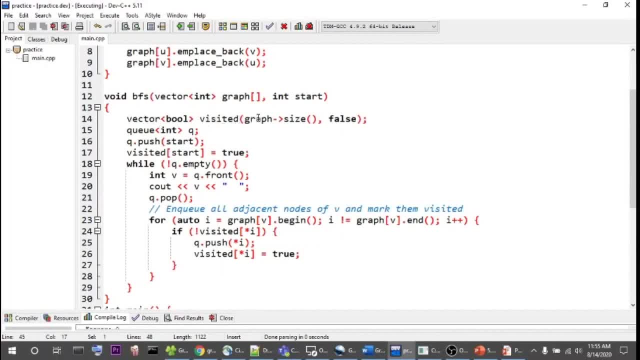 in this. i've created a listed vector which is equal to the number of vertices of the graph and initialized all of them in false. I create a queue and I push the start vertex in the queue and I mark the start vertex as listed. now I iterate until the queue is empty, so I pop the first element from. 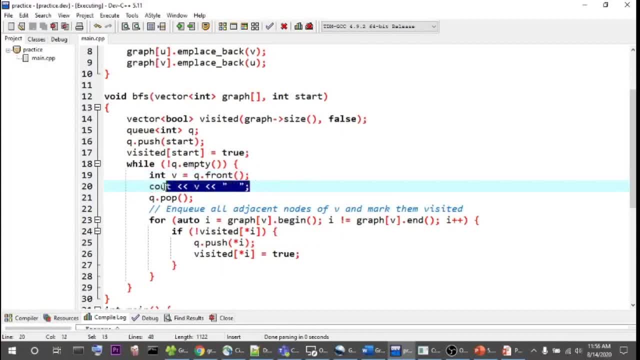 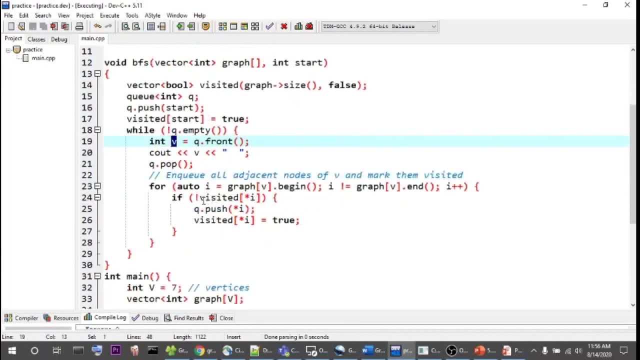 the queue and I print it. so this is where the bfs traversal is getting printed. then I check what are the adjacent nodes of this vertex and I check whether they have already been listed or not. if they're not listed, I push them in the queue and mark them as listed. so I keep doing that for. 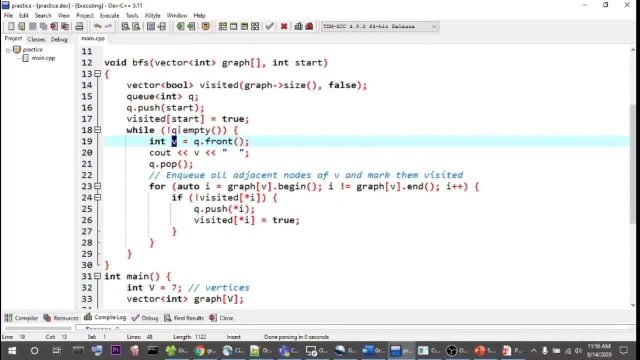 all the adjacent nodes and after this I pop the next element from the queue and I do the same thing. I keep doing this until the queue is not empty and at the end you will see that all the nodes will be printed. this will print the bfs traversal, if we check the output of this. so the 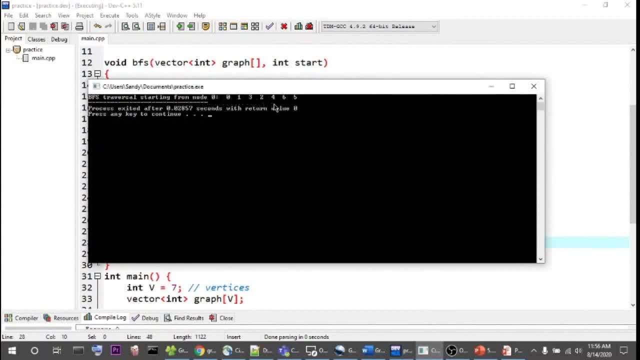 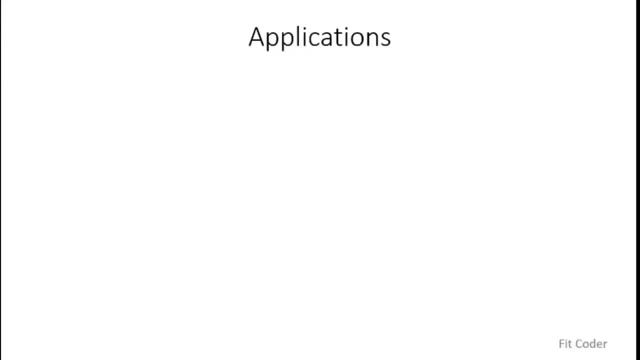 output is: bfs traversal, starting from node 0 is 0, 1, 3, 2, 4, 6, 5, so it is the same a, b, d, c, e, g, f. now, once you have understood how is bfs algorithm actually works, next important thing comes is: 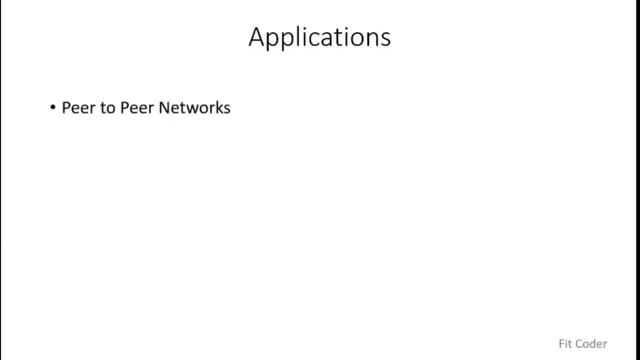 what are the applications of bfs and what are the applications of bfs and what are the applications of bfs and what are the applications that we have for bfs? so one of the applications that we have is peer-to-peer networks. so when we say peer-to-peer networks, we have new torrent, bit torrent, other torrent clients. 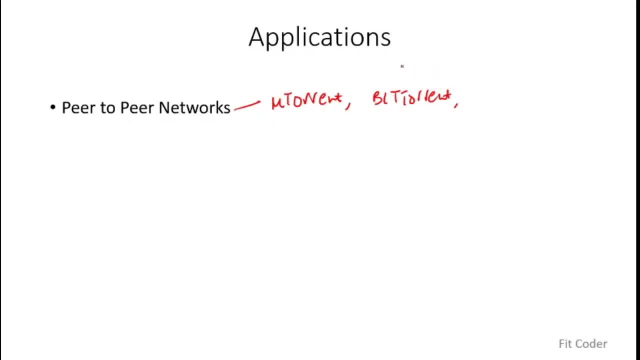 and all those kinds are there. so you will see in the status bar there. so it checks all the neighboring nodes, so the concept of neighboring that comes from bfs. so it checks what are the nodes that are adjacent to it and it can also check that. let's say you want to see what are the. 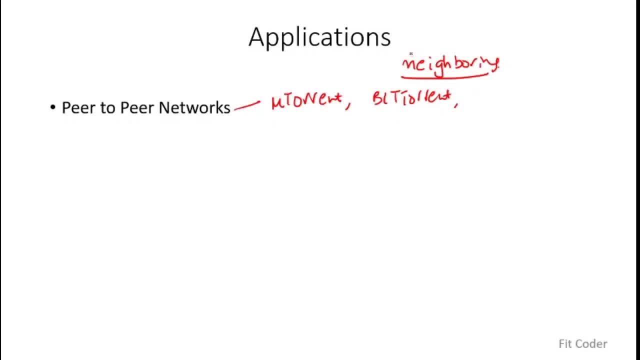 nodes that are at third level or second level. so this concept comes from bfs traversal and all these softwares that are there for peer-to-peer networks that rely on bfs traversals. another application that we have is for social networking sites. so let's say we have fb, we have linkedin, so in linkedin, 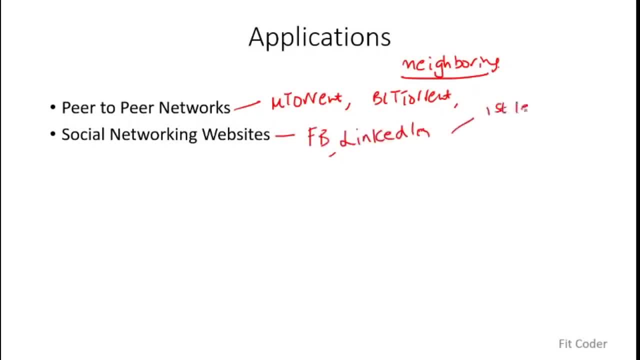 you might have seen that some people is at a first level of hierarchy. at some someone else is at second level of hierarchy, so how this level of hierarchy is maintained in terms of graph. so if you're friends with someone, let's say you are at person a, you're friends with b, then b is connected. 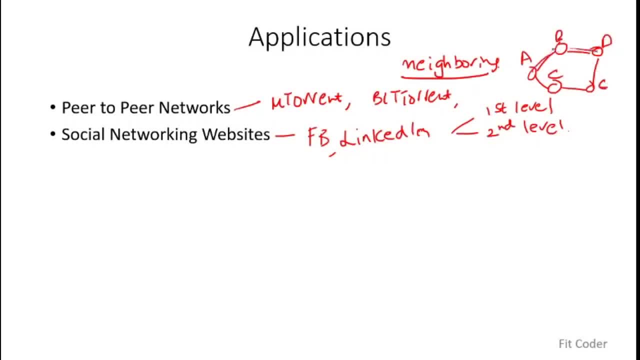 with d, so you are at second level, so you are at second level. so you are at second level, so you are at first level. so this level of information that is kept in graphs so that is used to display as the hierarchy information to you, so in social network websites, all these use bfs traversals a lot to. 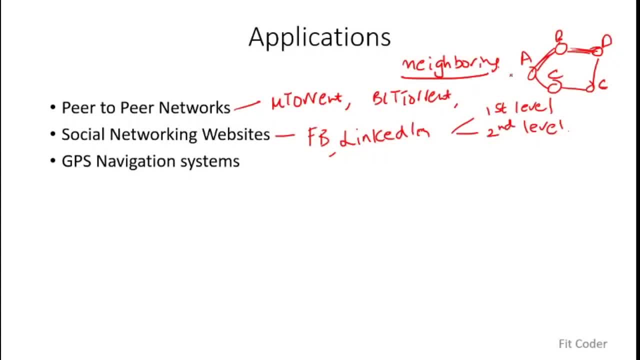 display this kind of information. the next application that we have is in gps navigation system. so in google's map or google search, if you have to find that, what are the nearest coffee shop that you have, let's say, at a point where you are located from one kilometer away? those navigation. 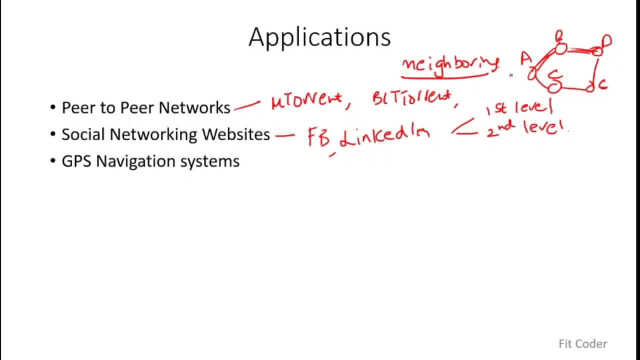 systems can use bfs traversals to check if the neighboring nodes have any of these coffee shops, a particular distance, so the distance can be the weight of the edge and then they can use this traverses to find in pathfinding, like we have discussed in games and other software where we 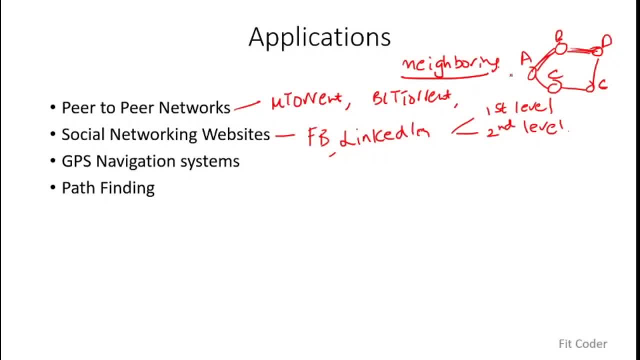 have to find the shortest distance to dc destination. but here we can also use dfs, so both of these algorithms can be used. then broadcasting in network. let's say you are in a peer-to-peer network or in a LAN network and you want to broadcast a message to all of your